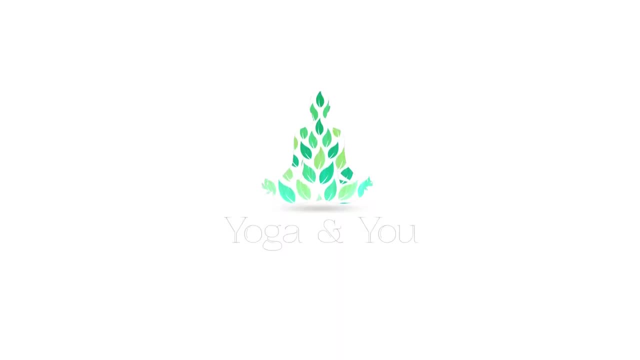 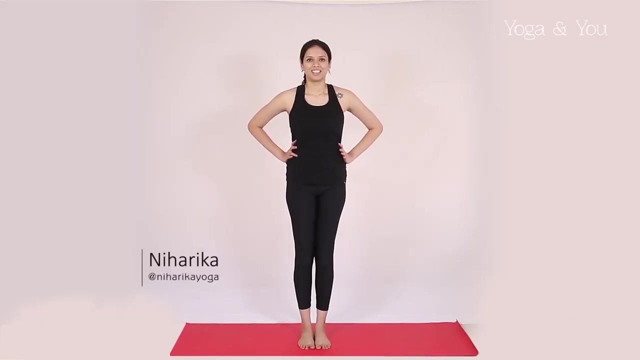 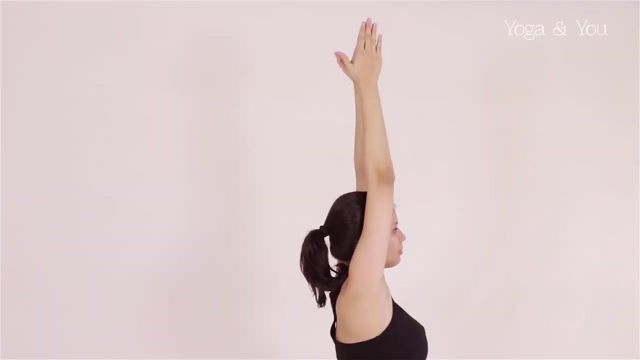 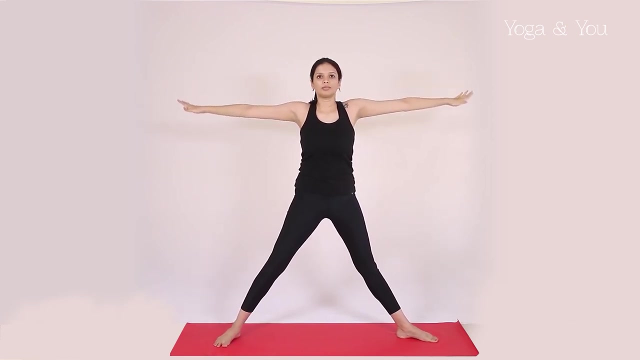 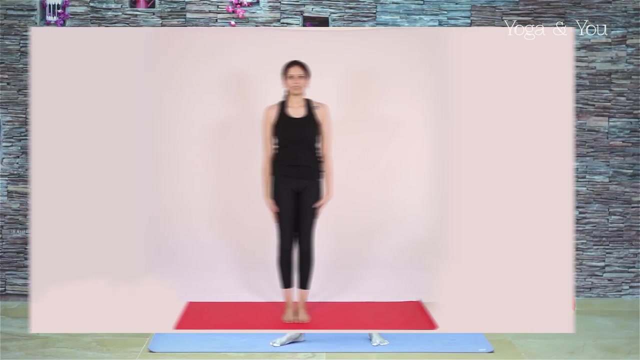 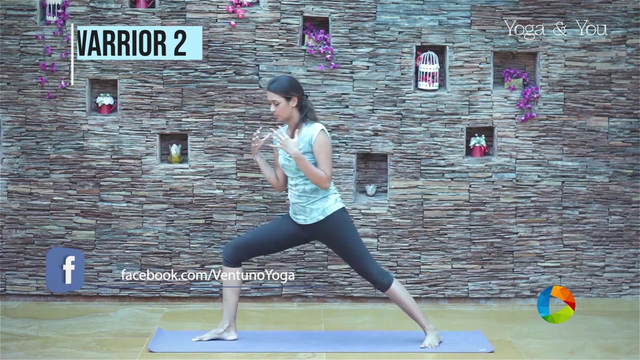 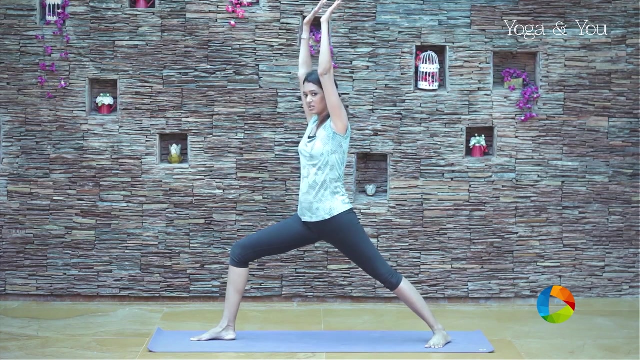 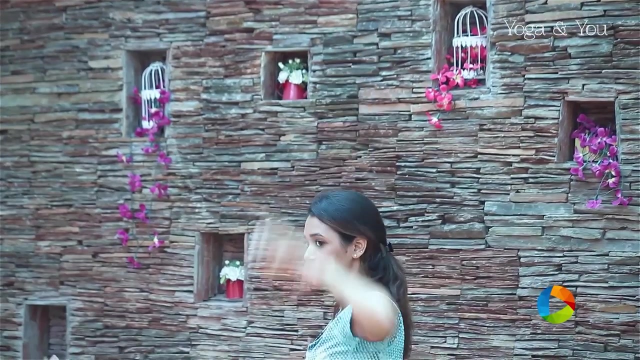 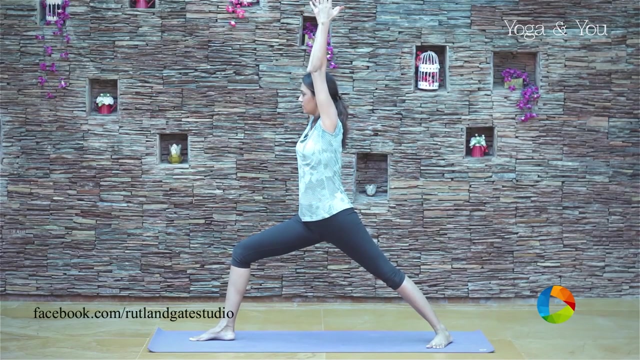 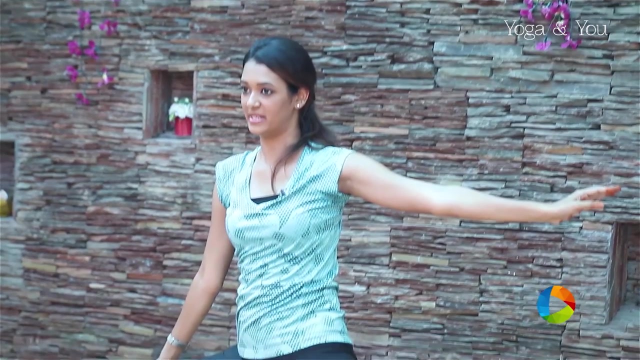 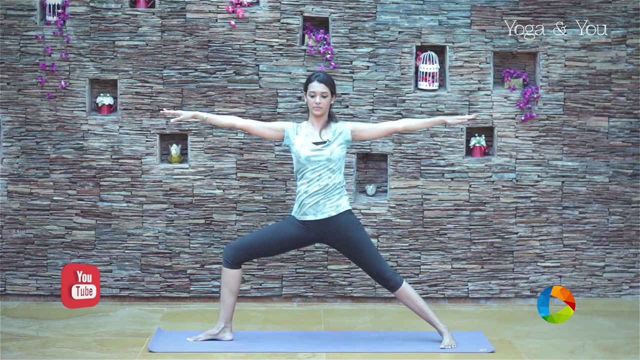 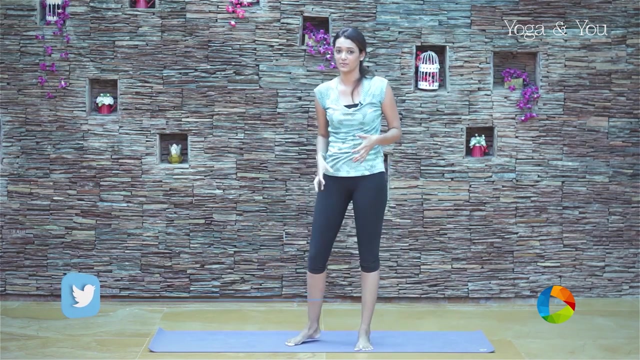 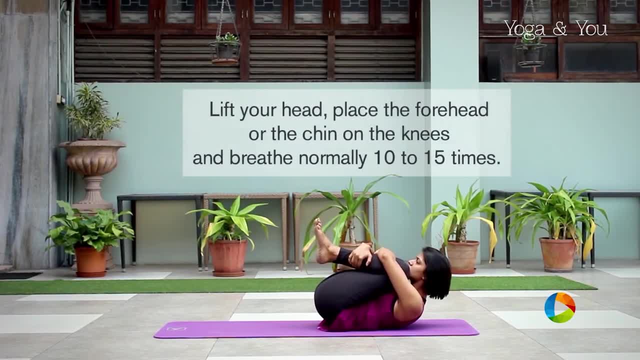 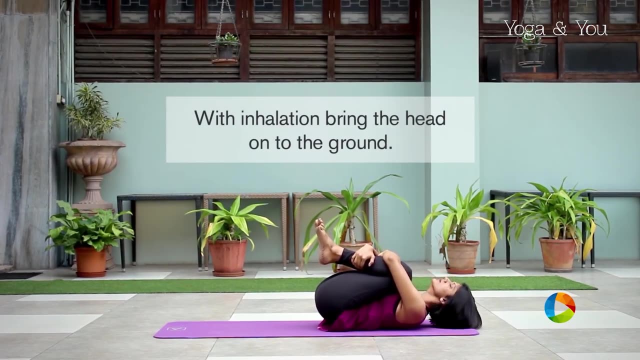 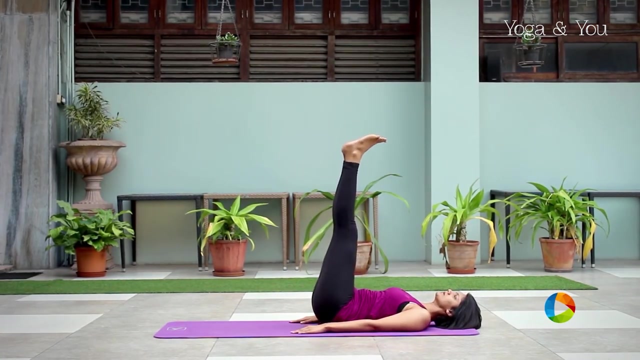 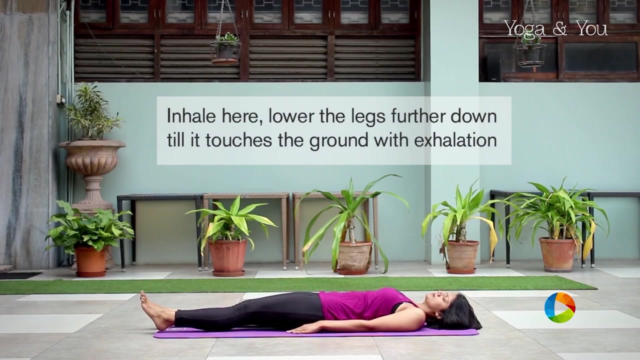 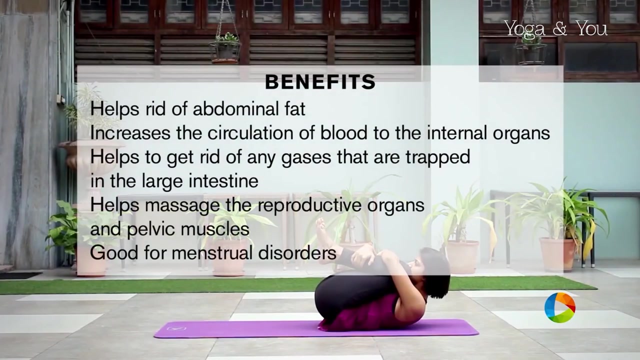 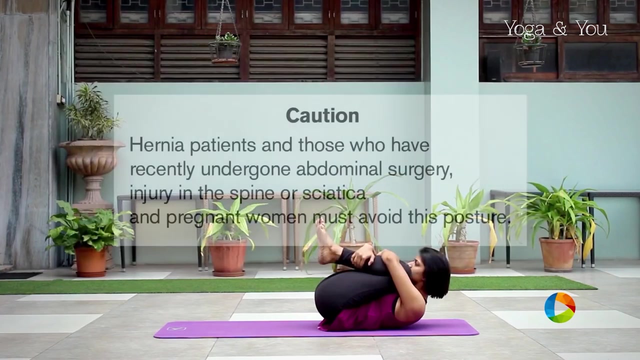 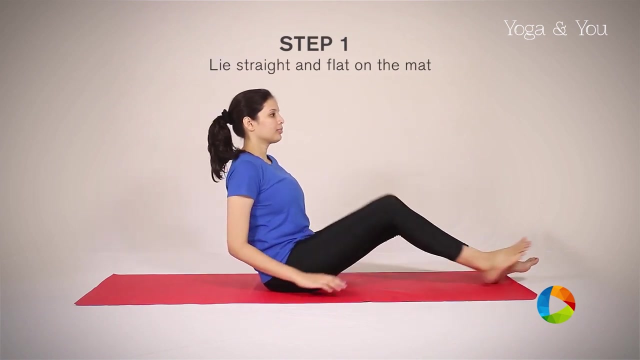 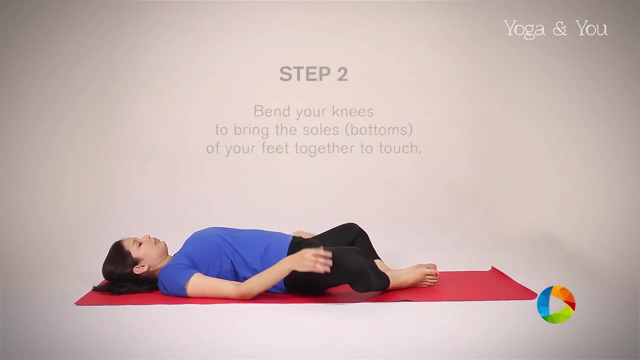 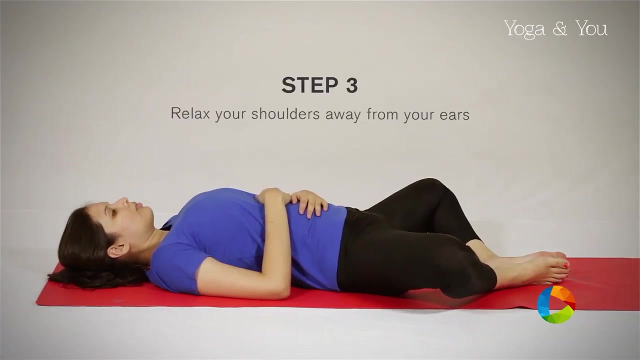 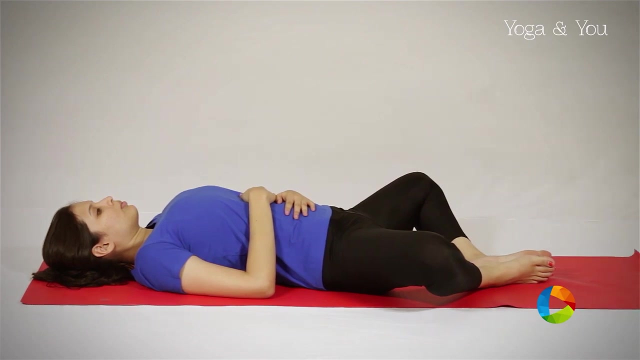 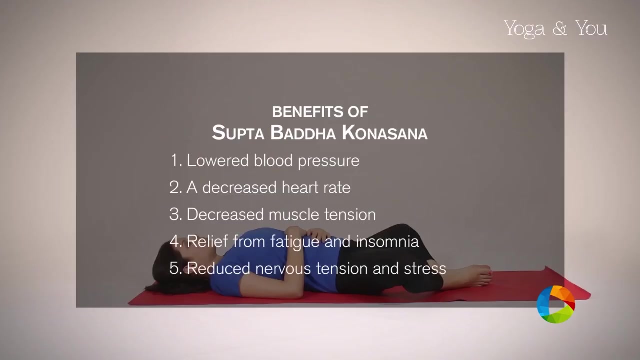 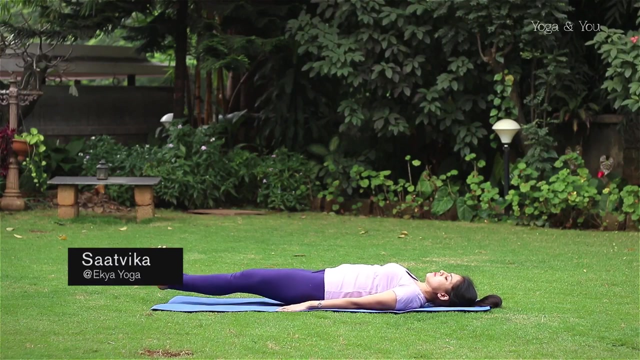 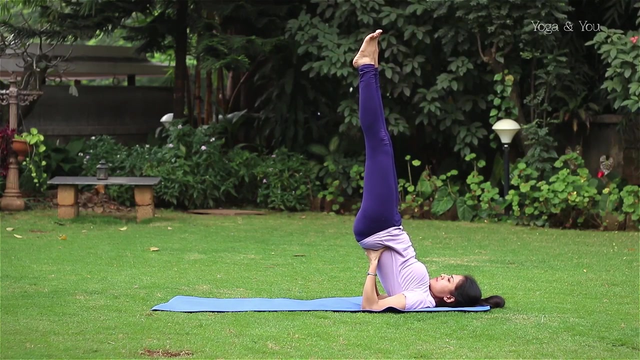 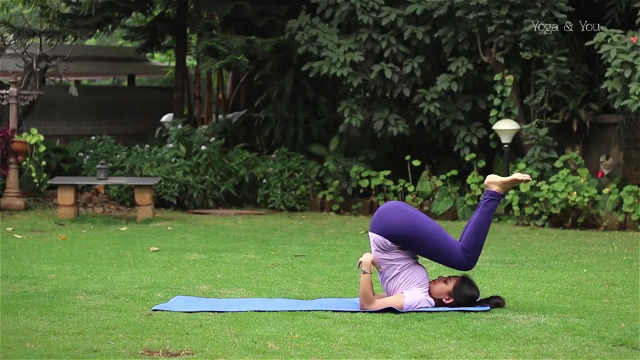 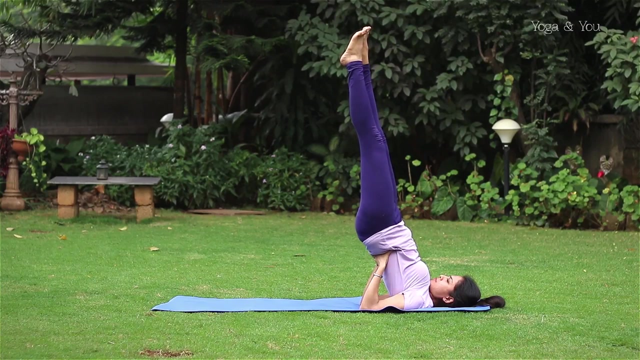 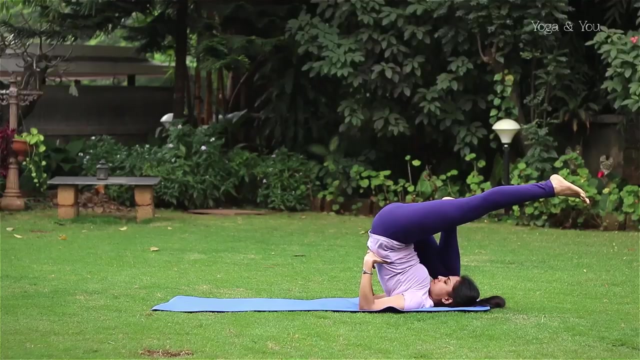 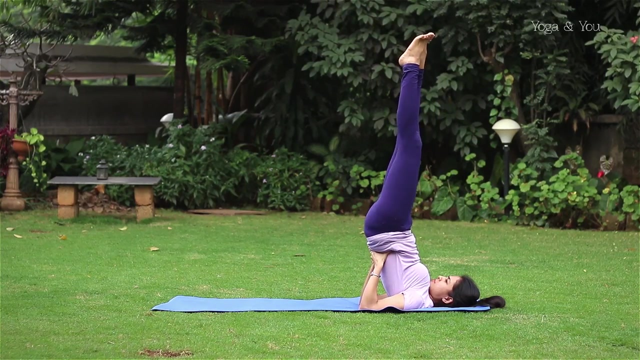 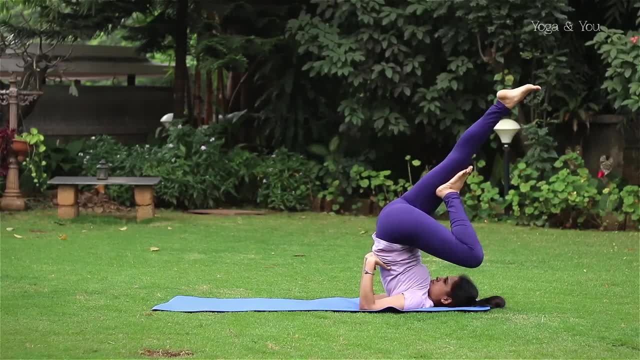 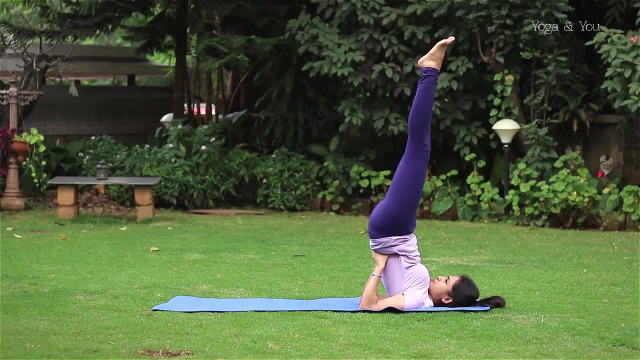 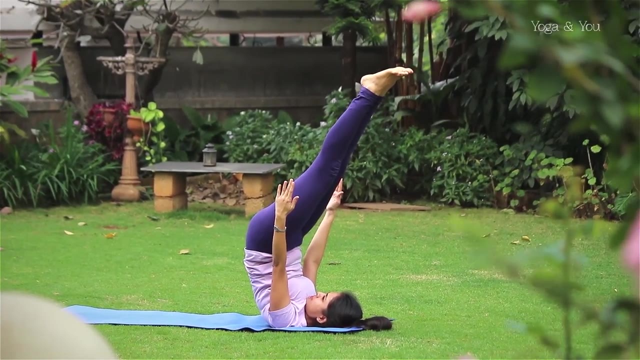 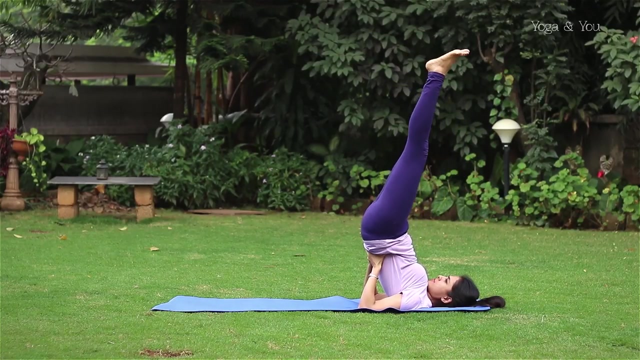 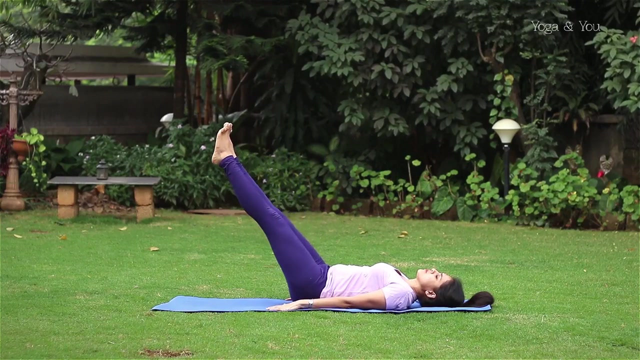 and release. coming back into regular sarvangasana from here, release one hand, bring it parallel to your legs and the other hand and stay in the unsupported sarvangasana to release. support your back, bring your legs above the head 45 degrees, roll out vertebra by vertebra and slowly bring the legs down.